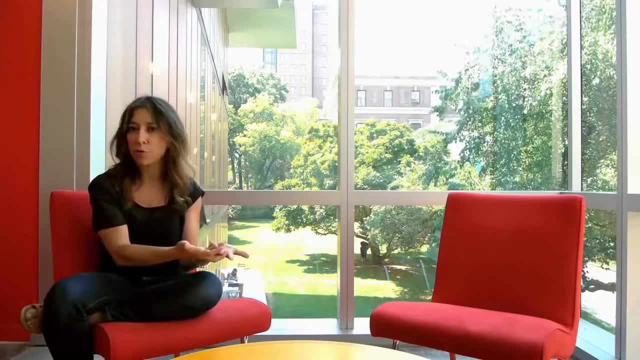 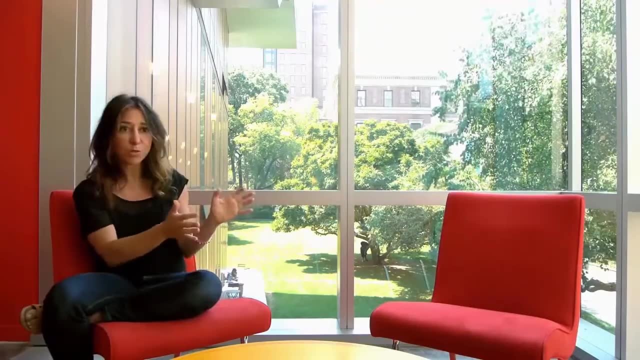 making a prediction, going to the observers to make an actual observation or building an experiment, and vice versa. Sometimes there are discoveries made with telescopes that we just didn't foresee, And then we have to go back to our pen and paper, back to the 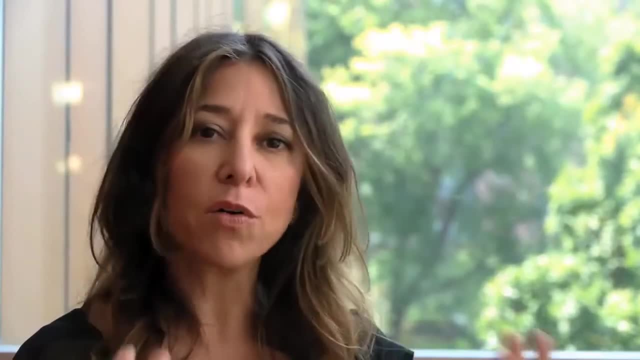 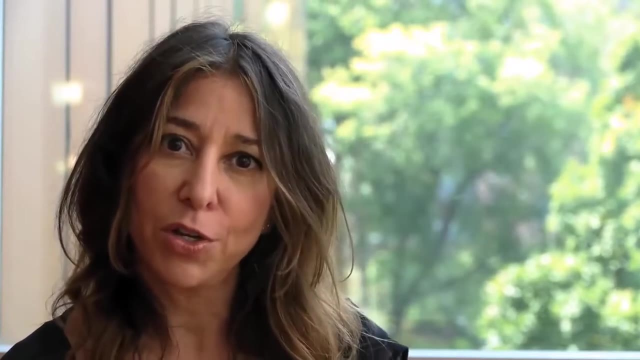 drawing board and figure out what did we miss and how could we not have predicted this phenomenon? And often it goes that way that we're trying to understand something And we're trying to think about ways to do it, And that's something we've seen in the 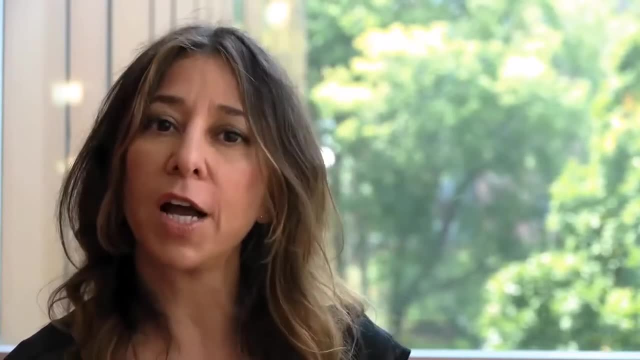 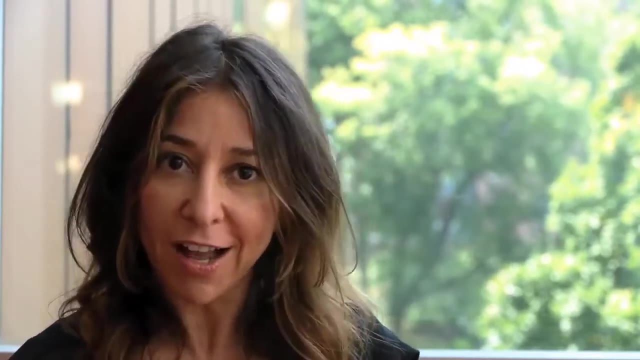 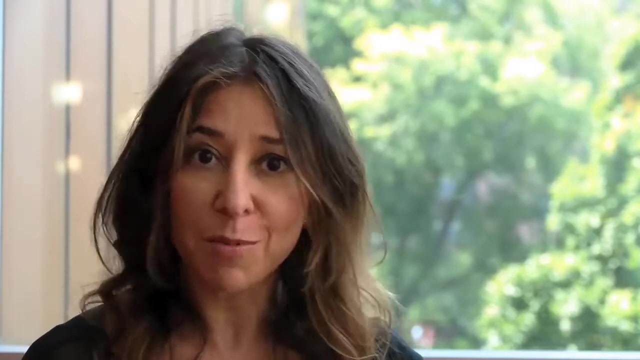 world but don't yet understand. So astrophysics draws from a lot of different kinds of study And I actually came to realize that this was this beautiful field kind of late. I was not interested in physics when I was a student. I was not one of those kids in the basement. 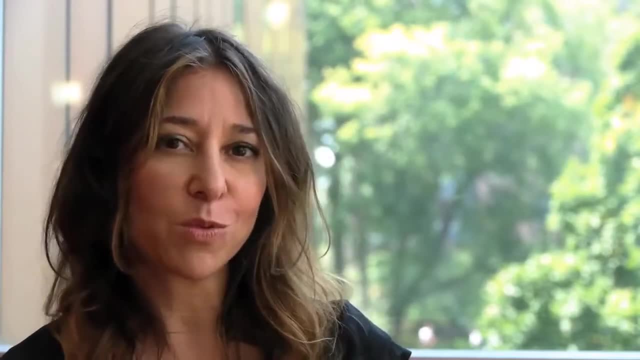 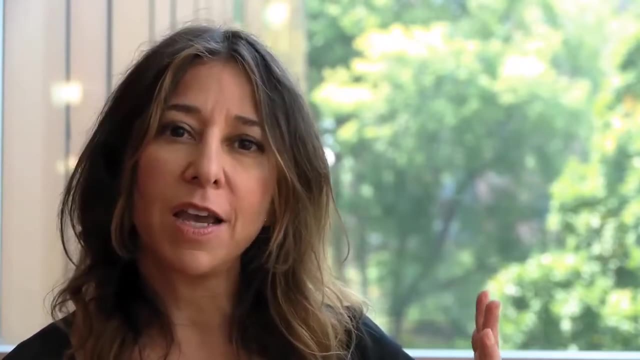 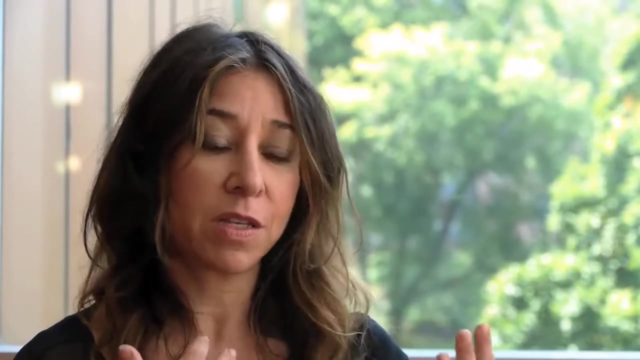 with the chemistry lab And I didn't understand or appreciate how elegant and beautiful science was until much later of mathematics, but I didn't recognize how rich and beautiful it was, and it wasn't until later when I understood that mathematics gives us this kind of it's a gift that connects 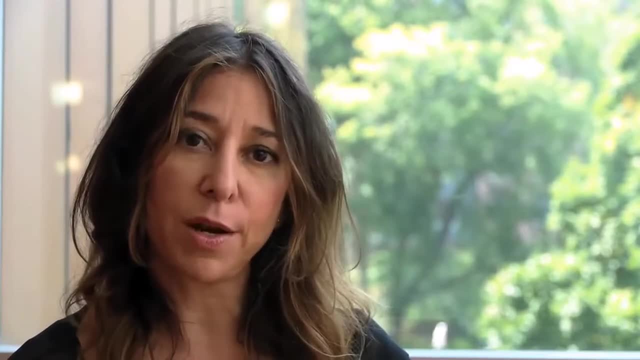 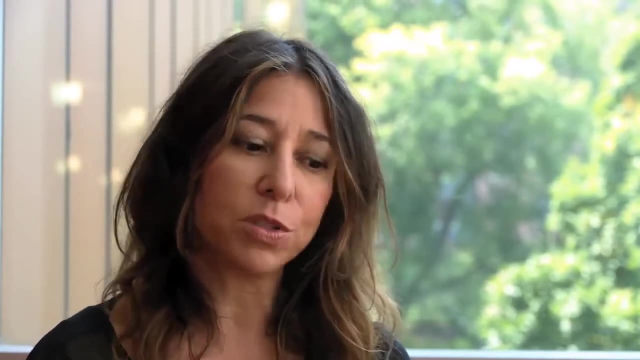 us to the natural world, that somehow, through mathematics, we're able to understand natural phenomena, and that's just remarkable, and that it's the same wherever you are in the world, and it's the same at the other side of the universe. you know, one plus one is still two. 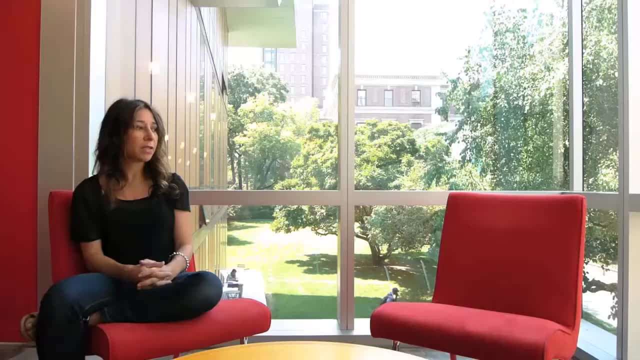 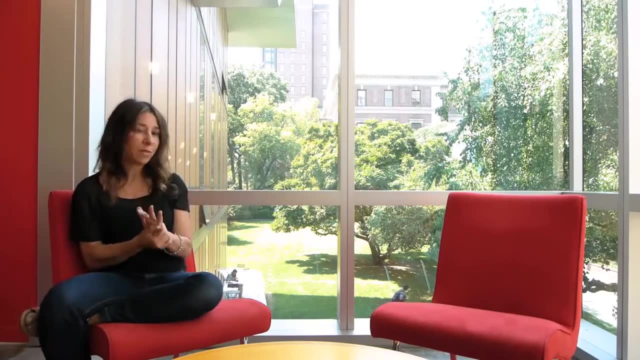 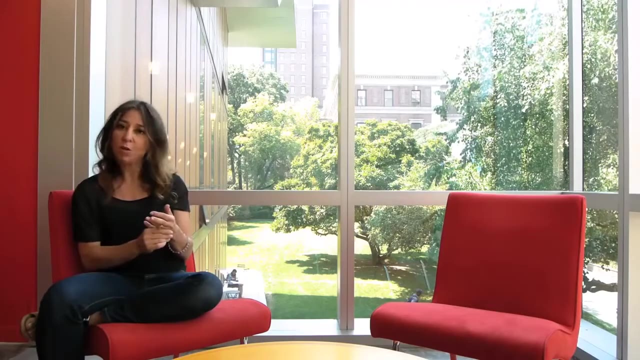 So there's something that connects all of us there. that seems really important, and when I discovered that in college, I became completely enamored of physics and math and astronomy and I started to study astrophysics and now I work on questions like: how did the universe 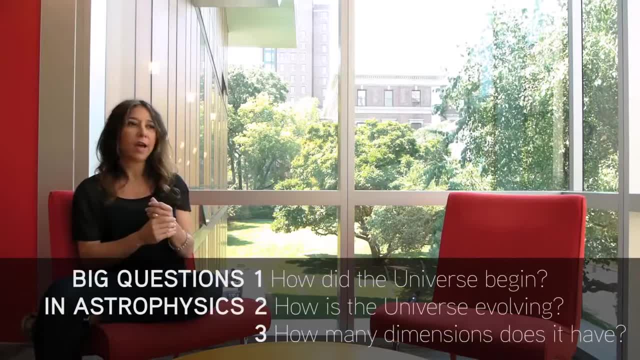 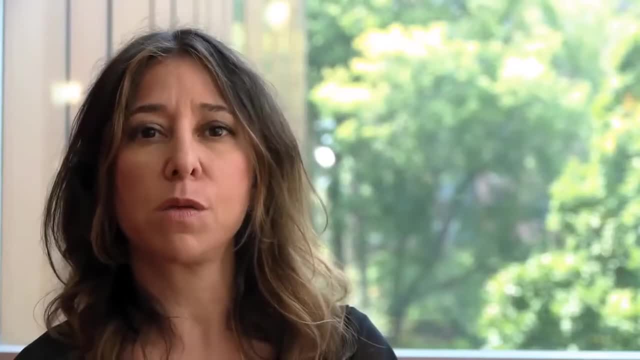 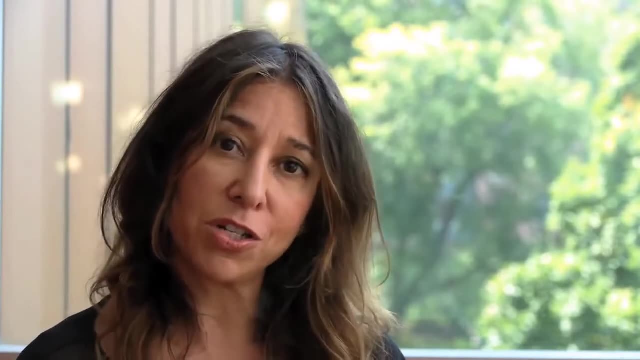 begin and how is it evolving? and how many dimensions are there? are there more than three dimensions in the universe? and what's the universe made of? Because the most important thing is the universe. The most important questions right now seem to be bound to an attempt to understand what 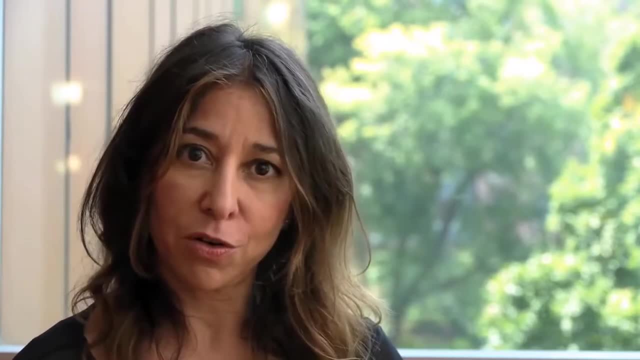 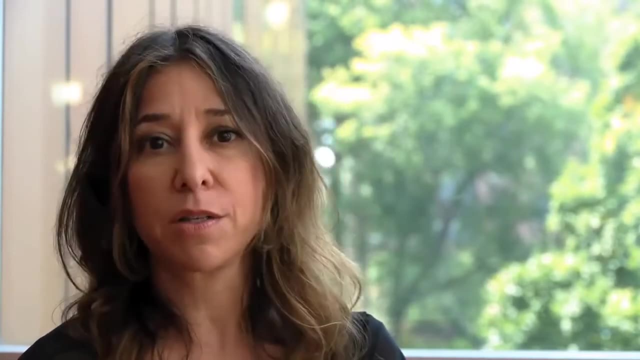 the universe is made of. because we've realized that most of the universe is in a form of matter and energy that we've never seen before, because it's literally dark. We cannot see it with our telescopes, but we know it's out there, because we can see the